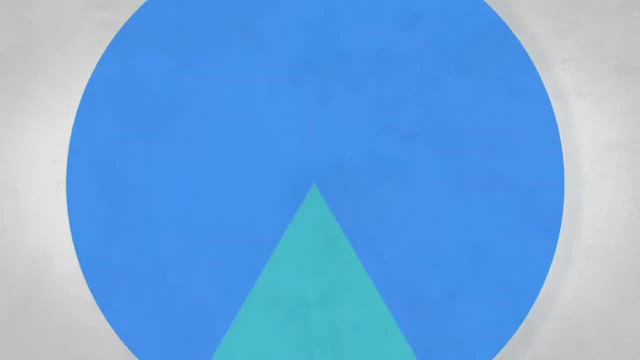 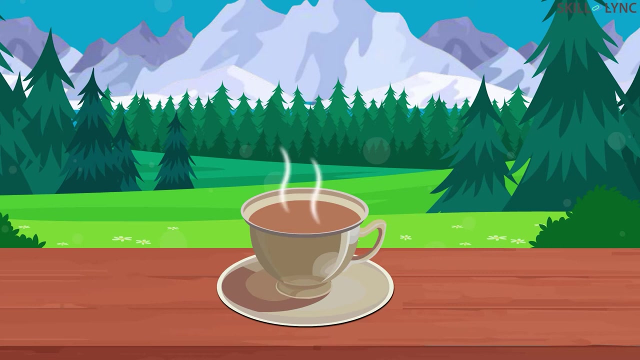 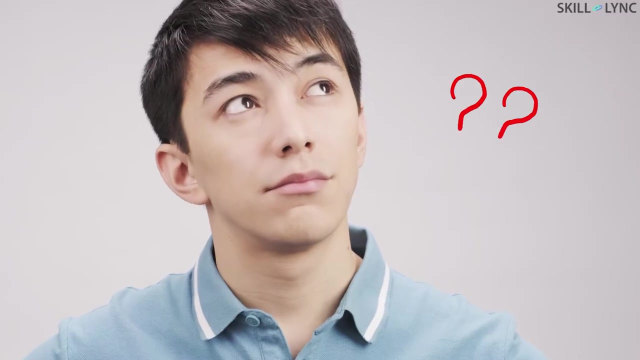 Hey guys, welcome back to our channel. We bet you guys enjoy drinking tea, coffee, hot chocolate, etc. However, when we leave a cup filled with tea in the open for some time, the tea gets cold. We all know how cold tea tastes, right? Do you guys wonder why this happens? Well, 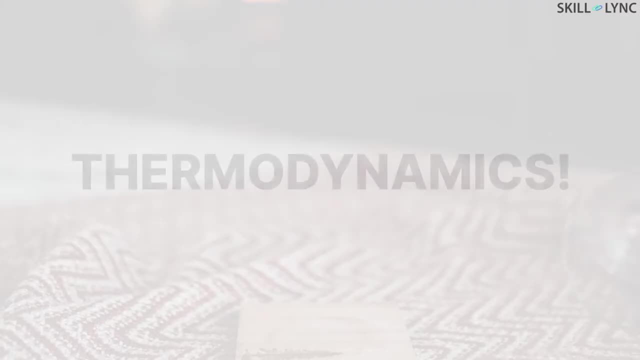 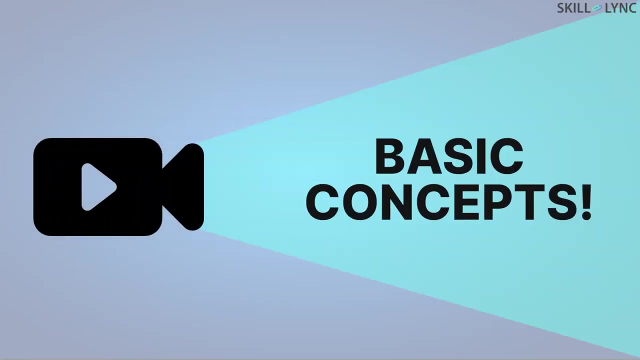 it's because of the transfer of energy from the tea to the surroundings. To understand this energy transfer, one must have a basic knowledge of thermodynamics. In today's video we'll talk about thermodynamics and some of its basic concepts in brief. We will be covering the 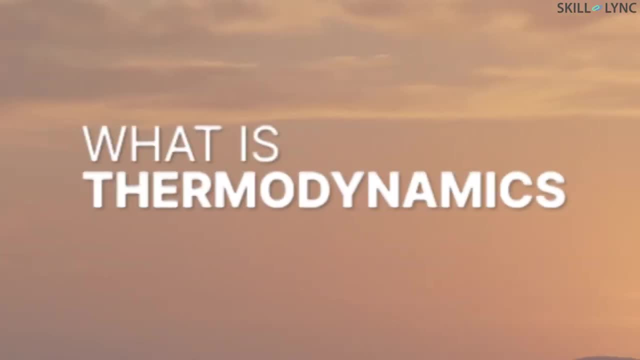 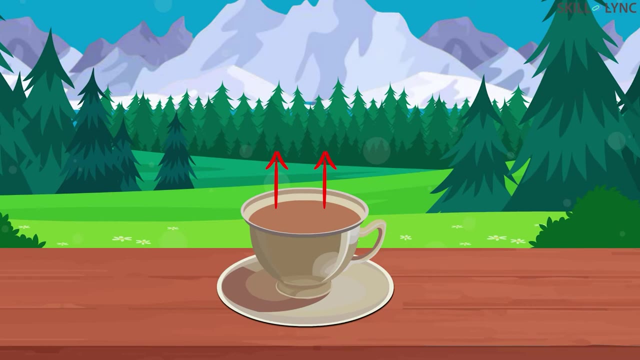 other topics in a bit more detail in some of the other videos. First of all, let's understand what thermodynamics is. It can be defined as a branch of science which deals with the relations among heat, work and properties of systems which are in equilibrium. It outlines the state 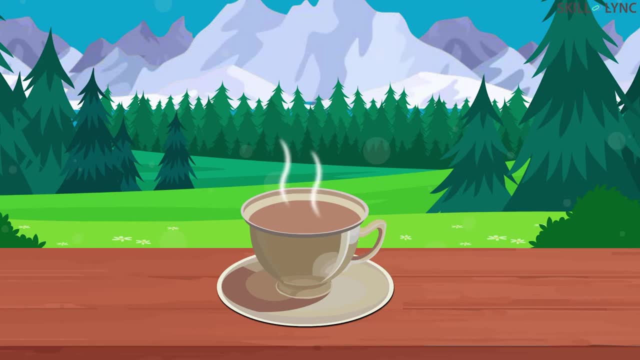 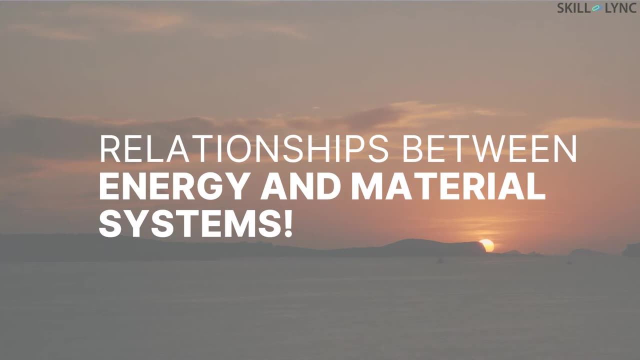 that is, the present condition of a system at a specific time and changes in state of physical systems. In simpler words, thermodynamics is the state of a system that is in a state of the branch of science which deals with the relationships between energy and material. 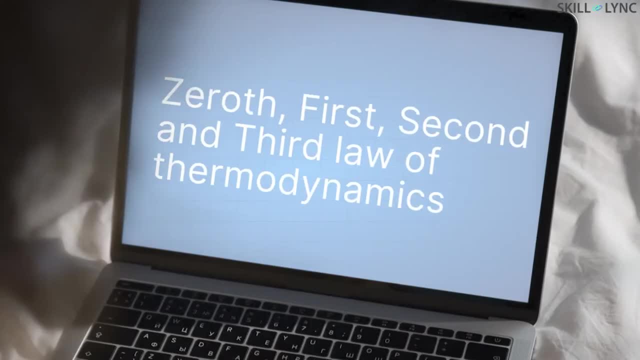 systems. The entire field of thermodynamics revolves around four laws, which are the first, second, third and the zeroth law of thermodynamics. The first law explains the concept of internal energy. The second law specifies the limit of converting heat into work and introduces the 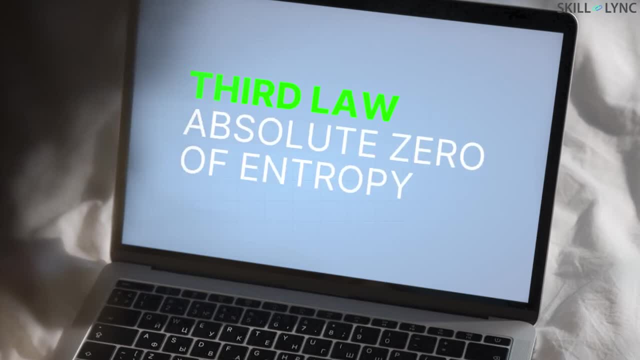 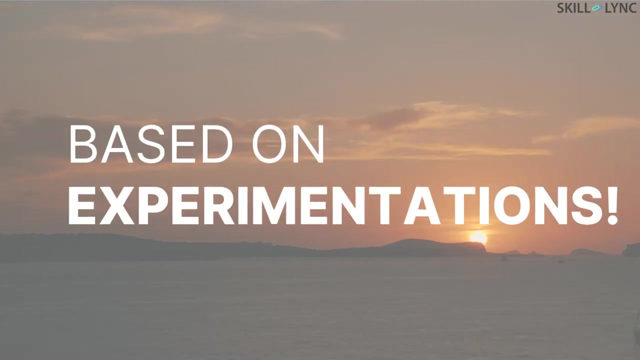 principle of increase of entropy. And the third law defines the absolute zero of entropy. The fourth law specifies the concept of temperature. We will cover all these laws and the terms related to them in our future videos. It must be noted that these laws are entirely based on. 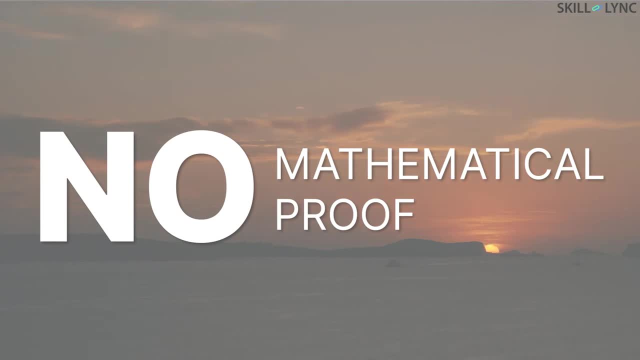 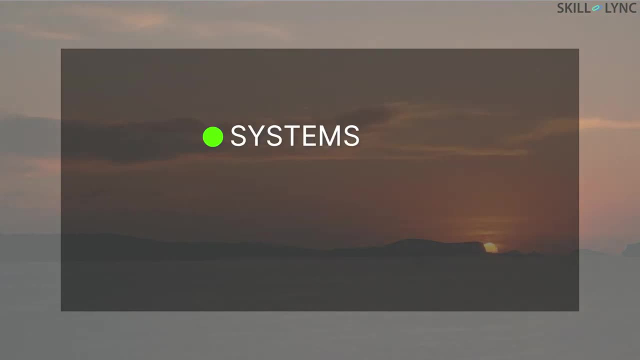 experimental observations and there is no actual mathematical proof for them. These laws are based on logical reasoning. During our study on thermodynamics, we will come across terms like systems, boundaries and surroundings, So let's talk about them. In thermodynamics, a system is: 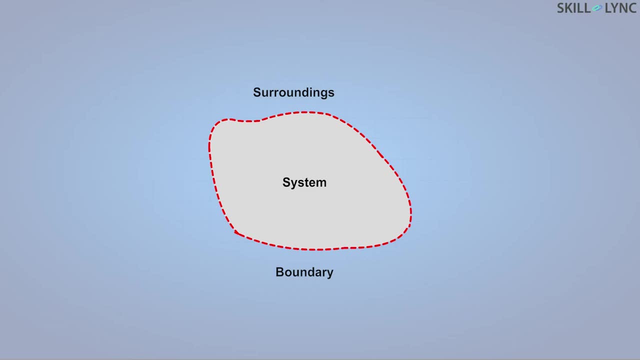 a finite quantity of matter or a given region of space which is a finite quantity of matter. So, under study, the actual or hypothetical cover enclosing the system is the boundary. This boundary may be stationary or non-stationary. Anything outside this boundary is the surroundings.